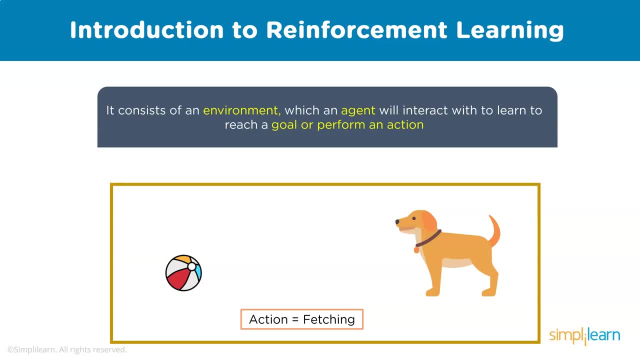 regression type model where we're looking at float numbers or we're trying to predict something or doing a reinforcement learning, where we're trying to guess the value of the stock market, where you have five point three, three, five dollars and thirty three cents. this is very a little bit. 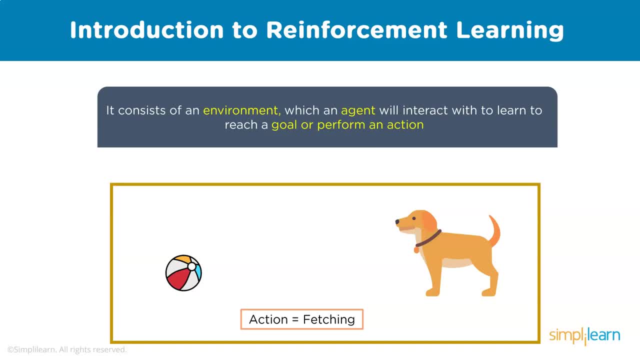 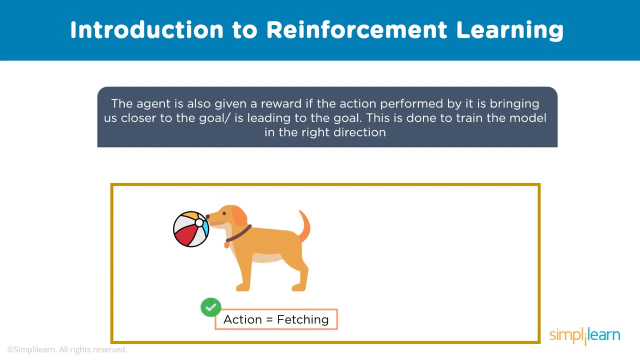 different and you'll see why Q learning is so powerful, but also where falls short. the agent is also given reward if the action performed by it is bringing, is closer to the goal, is leading to the goal. this is done to train the model in the right direction. you have a reward of a- hopefully a doggie cookie and action. 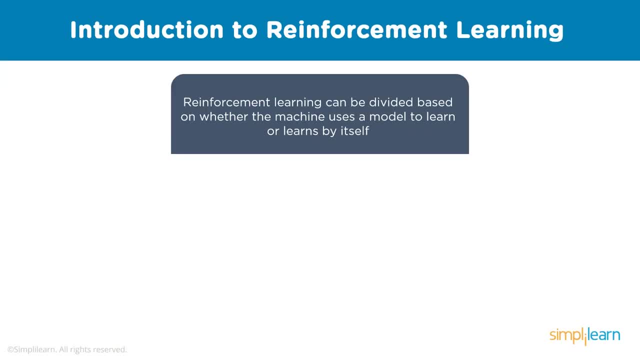 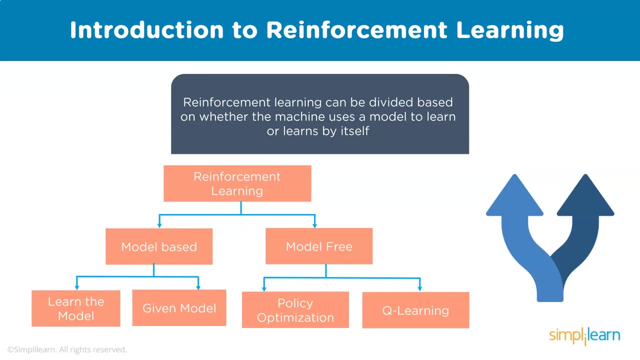 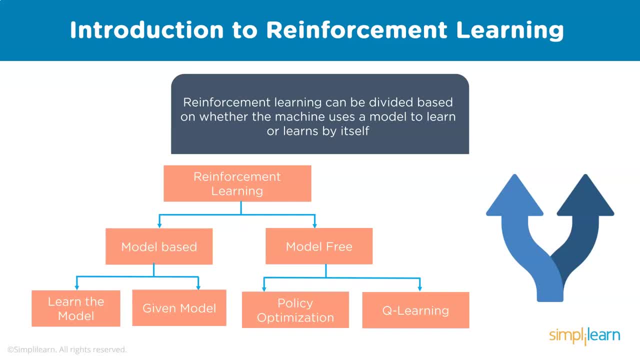 model given model and you can think of neural networks, I think are the most common right now used for reinforcement learning. there certainly are a lot of other options out there, but you have this black box and you go back and you send the error back up and it trains it based on how much of an error the error. 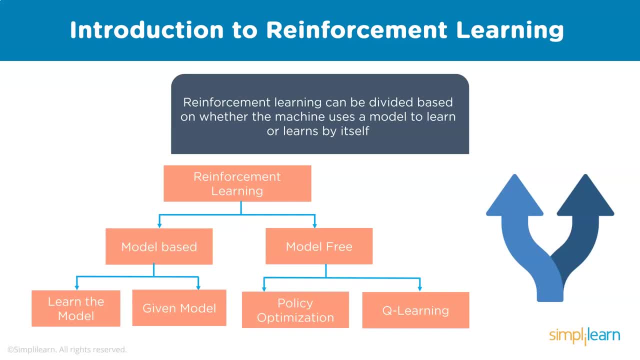 could be computed based on maybe a maximum reward subtraction or something like that. so the closer you get to the maximum reward, the better, and so we talk about a model free. you have your policy optimization and your Q learning, and this is kind of the cool thing about Q learning is it can do it's. 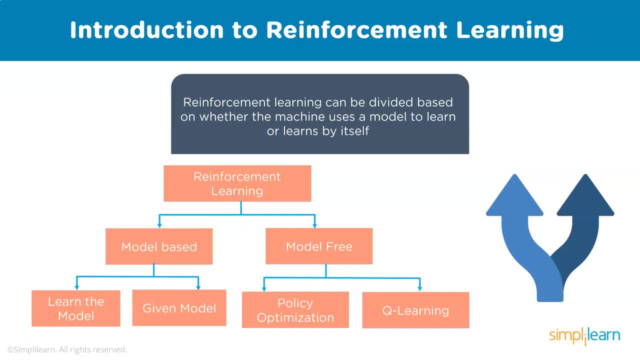 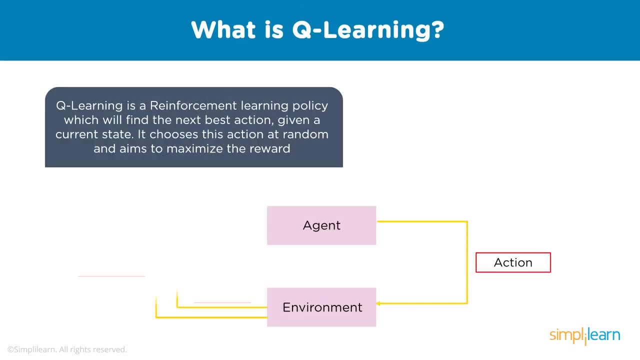 very powerful on certain things, making it very quick and easy to do a reinforcement learning. so what is Q learning? Q learning is reinforcement learning policy which will fill the next best action given a current state. it chooses this action at random and aims to maximize the and so you can see here's our standard reinforcement learning graph by now. if 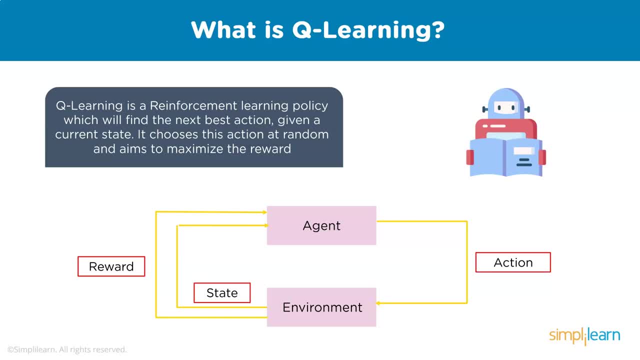 you're doing any reinforcement learning, you should be familiar with this. where you have your agent, your agent takes an action, the action affects the environment and then the environment sends back the reward or the feedback and the state is the new state, the agents in. where is it at on the chessboard? where is it at in? 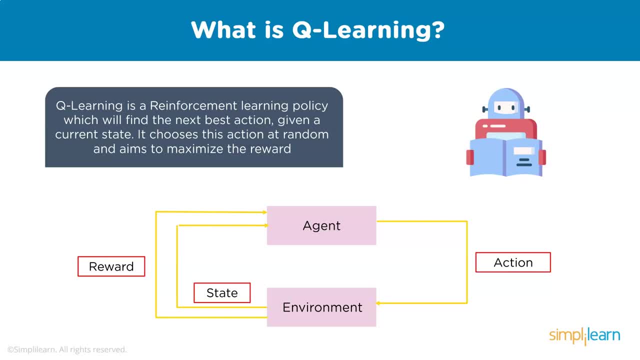 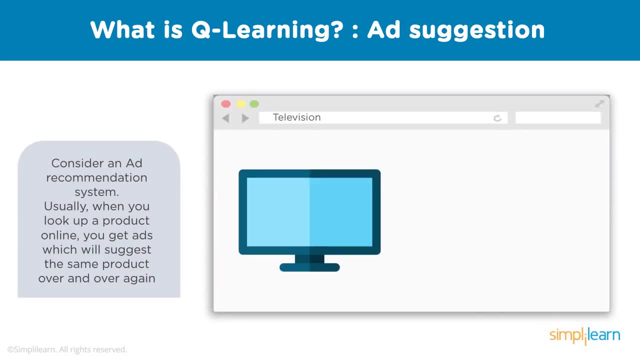 the video game. if your robots out there picking trash up off the side of the road, where is it out on the road? consider an ad recommendation system. usually, when you look up a product online, you get ads which will suggest the same product over and over again. using Q learning, we can make an ad. 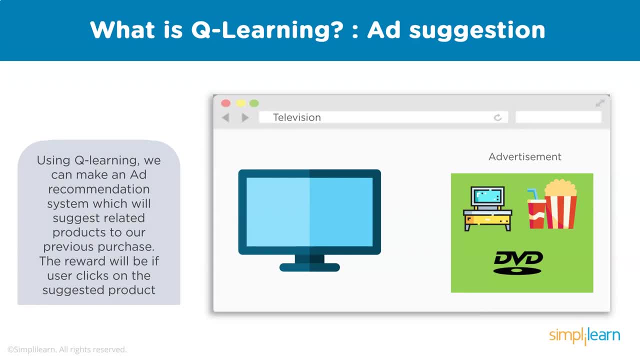 recommendation system, which will suggest related products to our previous purchase. the reward will be if user clicks on the suggested product and again you can see you might have a lot of product. if you click on the product that you should see something that doesn't on your web advertisement or your pages. but it's still not a float number. it's. 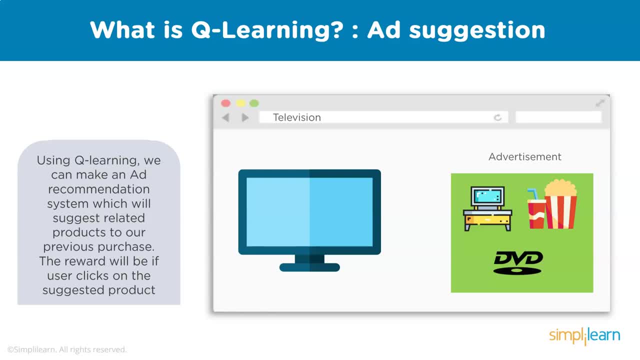 still a set number and that's something to be aware of when you're using Q-Learning. and you can see here that if you have a hundred people clicking on ads and you click on one of the ads, it might go in there and say, okay, this. 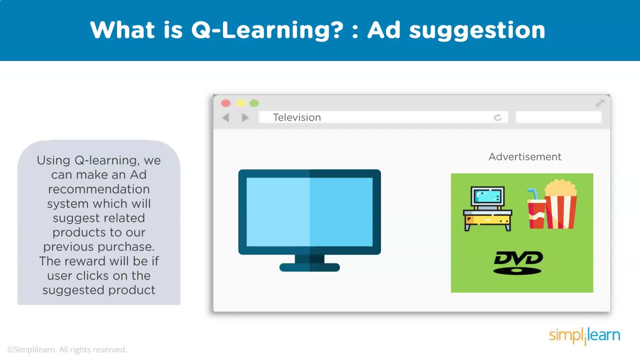 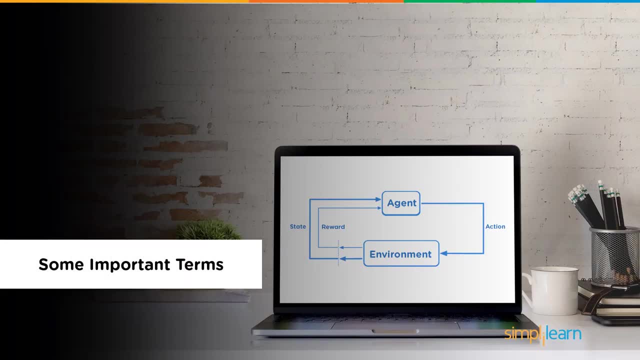 person clicked on this ad. what is the best set of ads, based on clicking on this ad or these two ads afterwards, based on where they are browsing? so let's go ahead and look at some important terms. when we talk about Q-Learning, we have states. the state S represents the current position of an agent in an. 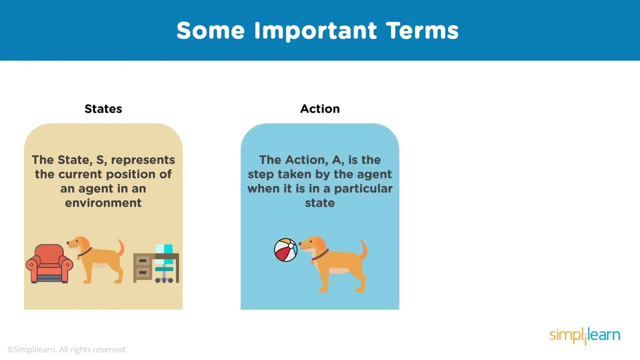 environment. the action. the action A is the step taken by the agent when it is particular state rewards. for every action the agent will get a positive or negative reward and again, when we talk about states, we're usually not with. when you're using a Q-table, you're not usually talking about float. 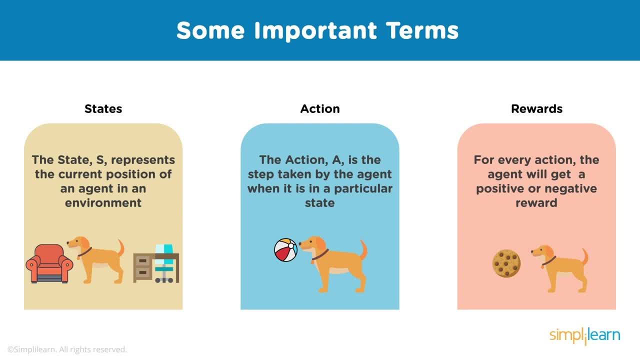 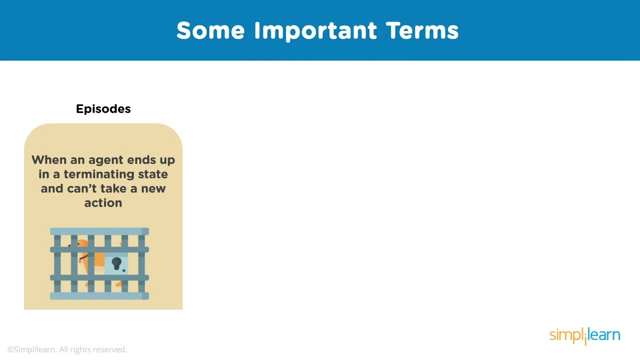 variables. you're talking about a set of ads and you're not usually talking about variables. you're talking about true, false- we'll take a closer look at that in a second- and episodes when an agent ends up in a terminating state and can't take a new action. this might be, if you're playing a video game, your character- 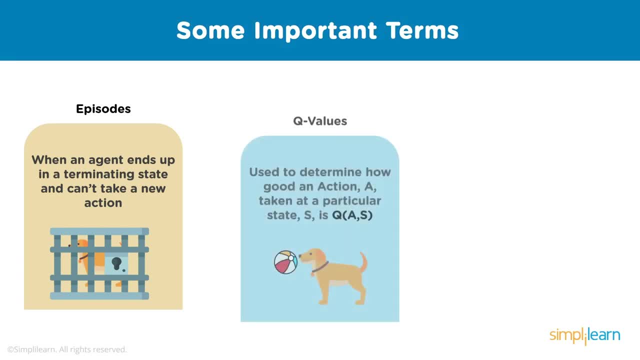 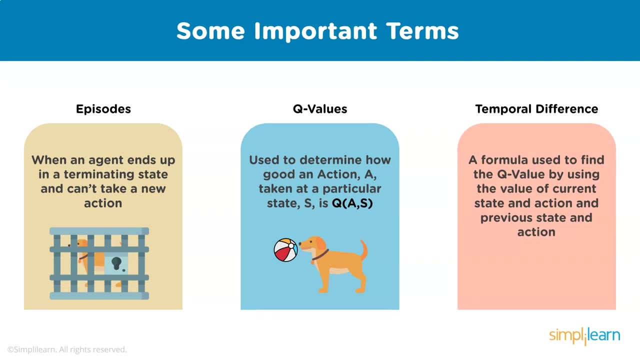 stepped in and is now dead, or whatever. Q-values used to determine how good an action A taken at a particular state. S is Q A of S and temporal difference. a formula used to find the Q-value by using the value of the current state and action and previous state and action and various. I mean there's Bellman's equation. 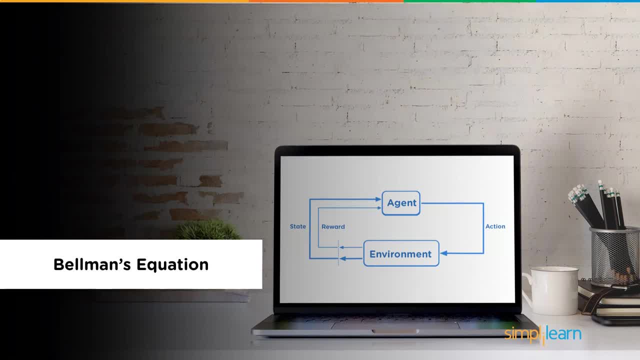 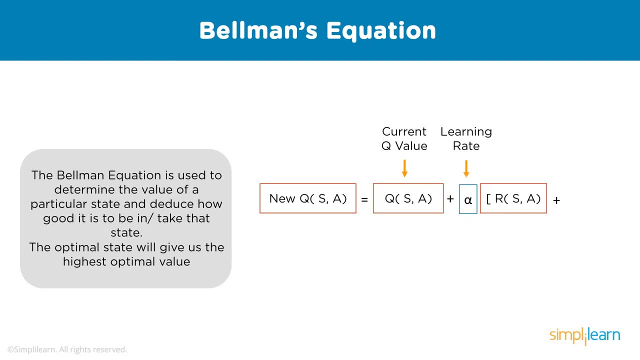 which basically is the equation that kind of covers what we just looked at in all those different terms. the Bellman equation is used to determine the values of a particular state and deduce how good it is to be in take that state. the optimal- the optimal state will give us the highest optimal value factor influencing. 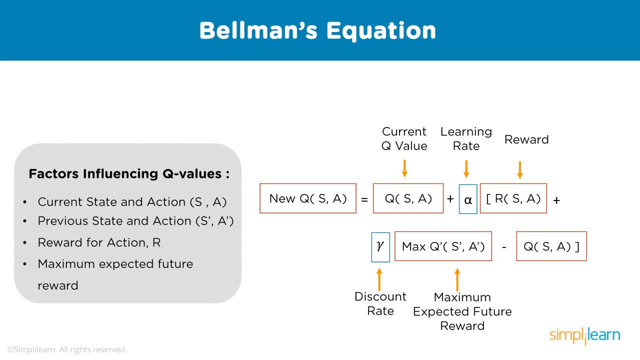 Q-values the current state and action. that's your SA. so your current state in your action. then you have your previous date in action, which is your S, I guess, prime. I'm not sure how they how they reference that S prime, a prime. so this is what happened before. then you have a reward for action, so you have your R. 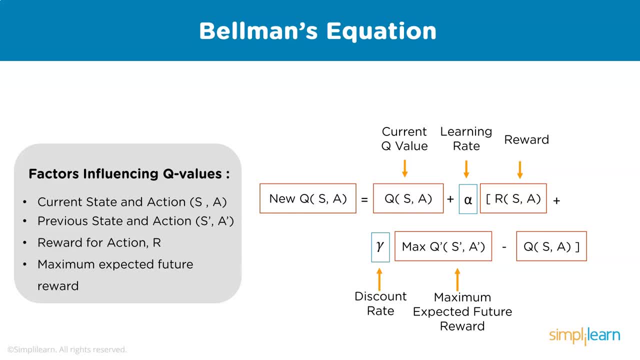 reward and you have your maximum expected future reward and you can see there's also a learning rate put in there and a discount rate. so we're looking at these just like any other model. we don't want to have an absolute final value on here. we don't want it to, if you do absolute. 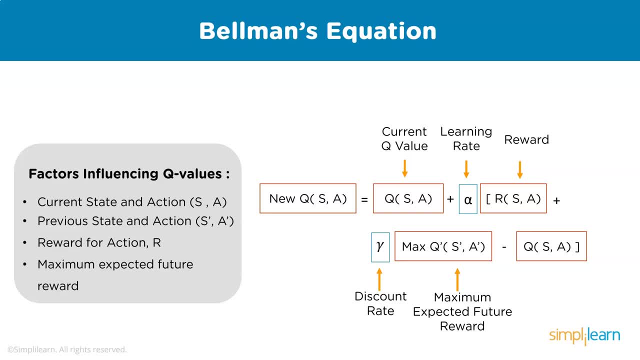 values instead of taking smaller steps. you don't really have that approach to the solution. you just have a jump and then pretty soon, if you jump one solution out, that's what's going to be the new solution, whichever one jumps up really high first, kind of ruining the whole idea of doing a random selection. 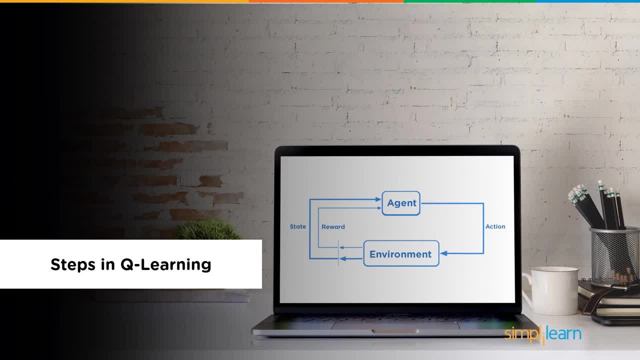 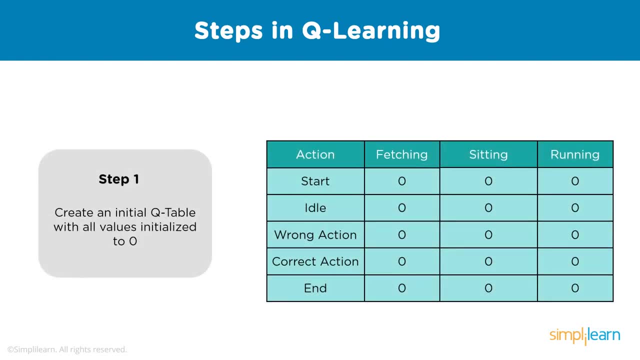 you can see that's what's going to be the new solution, whichever one jumps up really high first, kind of ruining the whole idea of doing a random selection. I'll go into the random selection just a second. steps in Q learning. step one: create an initial Q table with all values initialized to zero. again we're. 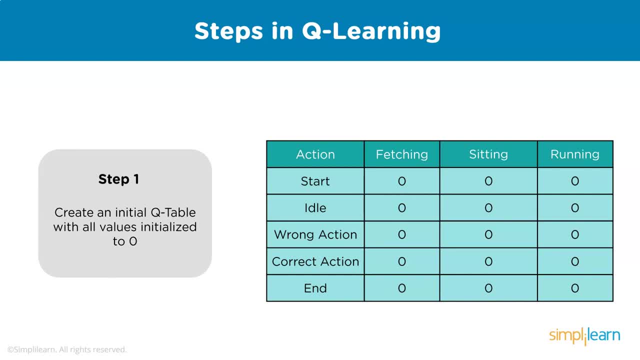 looking at zero one. so are you? you know, here's our action. we start, we're an idle, we took a wrong action, we took a correct action in int and then we have our actions: fetching, sitting and running. of course, we're just using the dog example and choose an action and perform it, update values in the table and, of course, 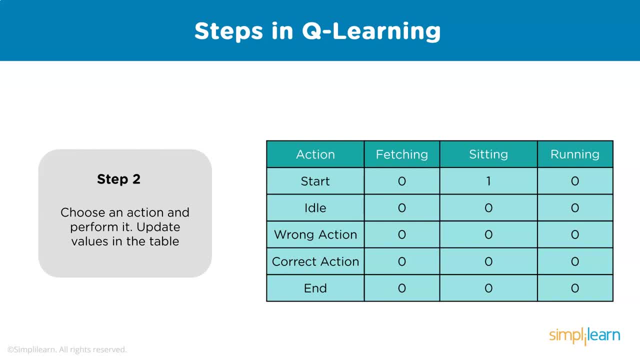 when we're choosing an action, we're going to kind of do something random and just randomly pick one, so you start out and you sit and you have. then, then, depending on that action you took, you can now update the value for sitting after you start, from start to sitting, get the value of the reward and 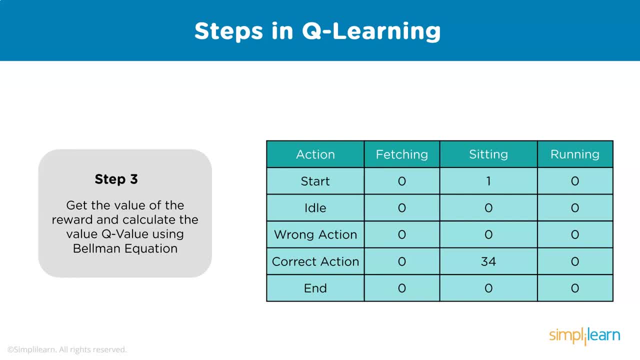 calculate the value, the value, Q value, using the Bellman equation. and so now we attach a reward to sitting and we attach all those rewards, we continue the same until the tables filled with or an episode ends. and my mission is going to come back to the random side of this, and there's a few different formulas. they 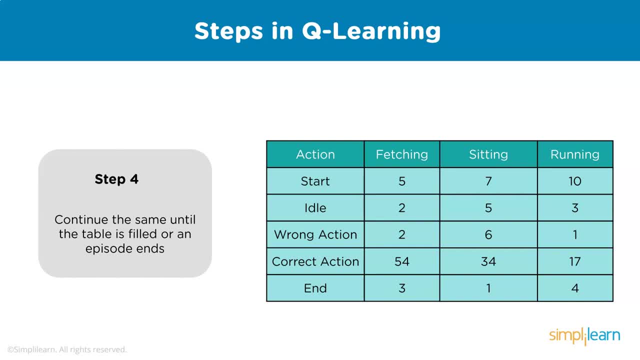 use for the random set up to pick it. I usually look whatever Q model I'm using do their standard one because someone's usually gone in and done the math for the optimal spread. but you can look at this: if I have, running has a reward of 10. 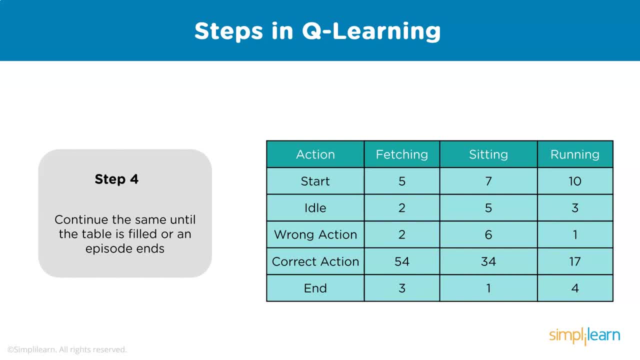 sitting as a reward of seven. fetching has a reward of five, just kind of without doing like a means to using the bell curve for the means value. and, like I said, there's some math you can put in there to pick so that you're more like, so that running has even a higher chance. but even if you were just going to do an 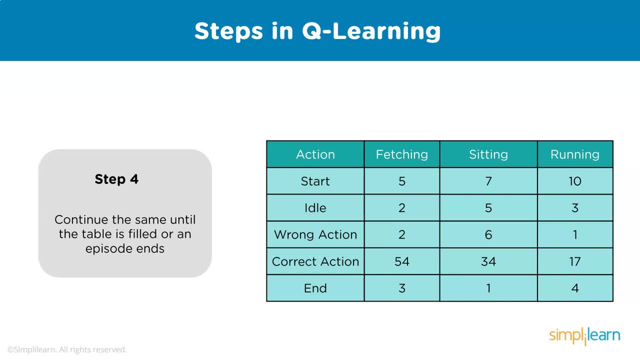 average on this. you could do an average, a random number, by adding them all together. so you get 10 plus 7 plus 5 is 22. you do 0 to 22 or 0 to 21, but 1 to 22, 1 to 5 would be fetching, and so forth, you know. 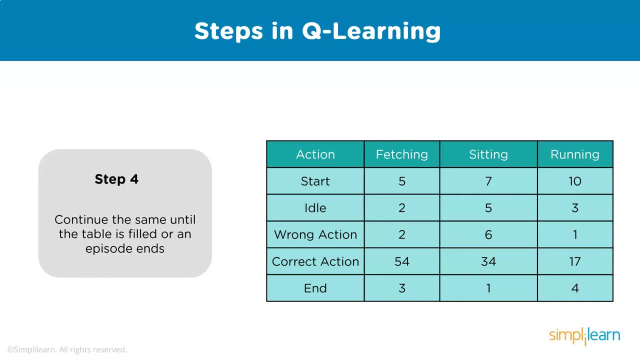 the last 10. so you can just look at this: as what percentage are you going to go for that particular option? and then that gets your random setup in there, and then, as you slowly increment these up, you see that if you're idle, where's one? here we. 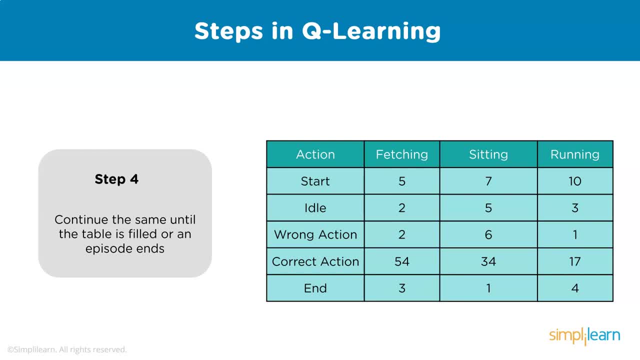 go sitting at the end. if you're at the end of wherever you're at sitting gets a reward of one. where's a good one on here, Oh, wrong action, running for a wrong action gets almost no reward. so that becomes very, very less likely to happen, but it still. 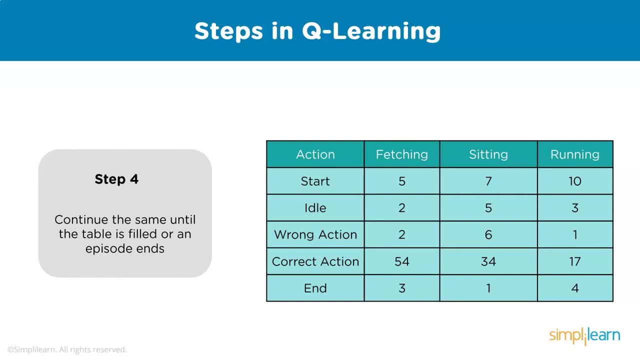 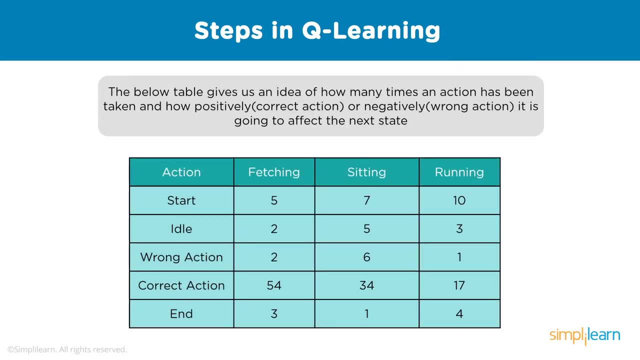 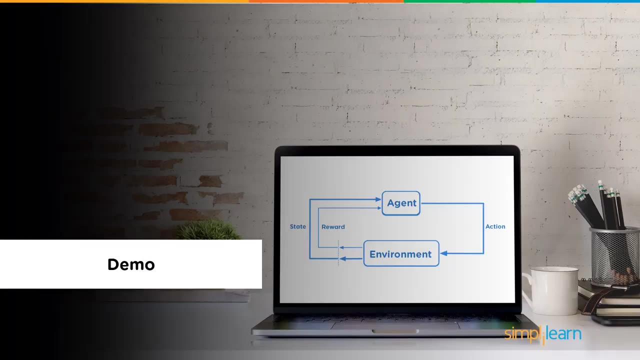 might happen, it still might have a percentage of coming up, and that's where the random programming and Q learning comes in. the below table gives us an idea of how many times an action has been taken and how positively correct action or negatively wrong action- it is going to affect the next state. so let's 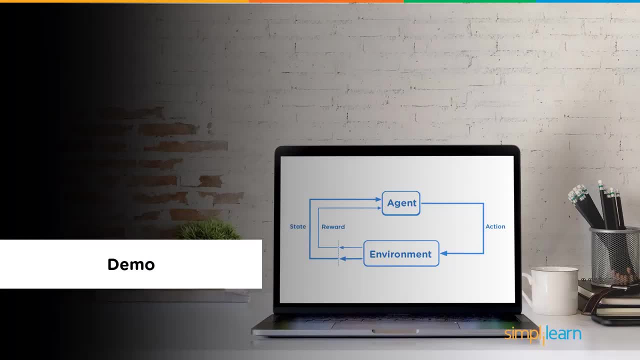 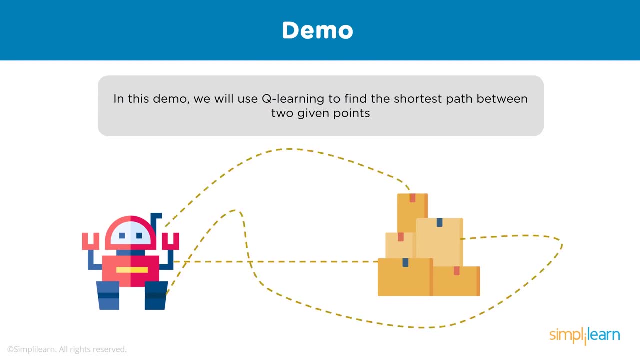 go ahead and dive in and pull up a little bit of the table, and let's go ahead and pull up a little piece of code and see what this looks like in Python. in this demo, we'll use Q learning to find the shortest path between two given points. 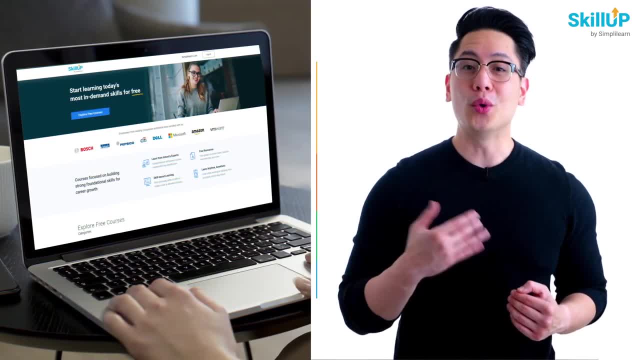 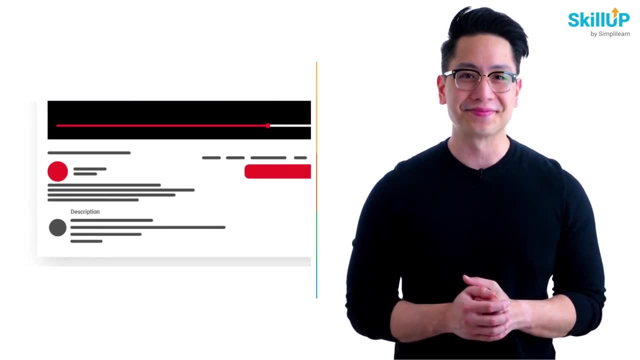 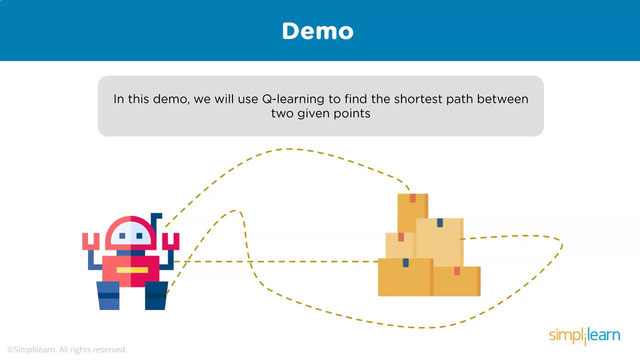 if getting your learning started is half the battle? what if you could do that for free? visit skill up by simply learn. click on the link in the description to know more. if you've seen my videos before, I like to do it in the Anaconda Jupiter notebook. 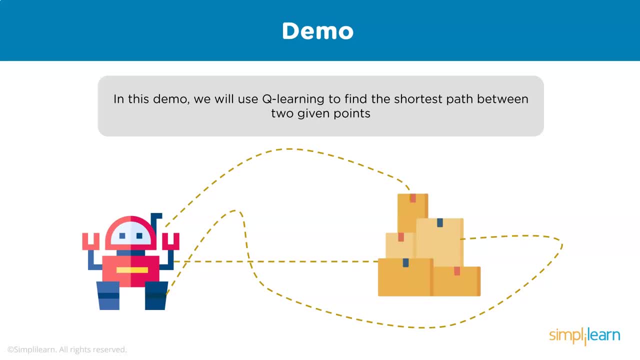 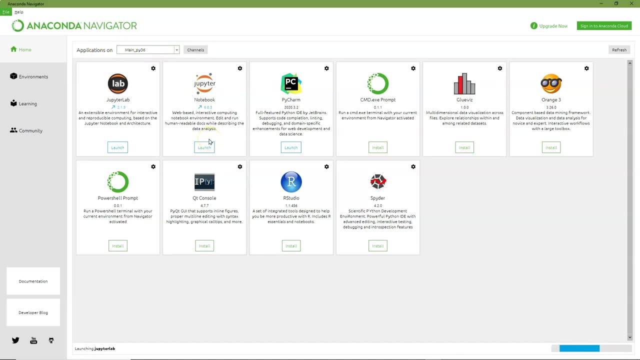 setup, just because it's really easy to see and it's a nice demo. and so here's my Anaconda, this one. I'm actually using Python 3 6 environment that I set up in here, and we'll go ahead and launch the Jupiter notebook on this, and once we're. 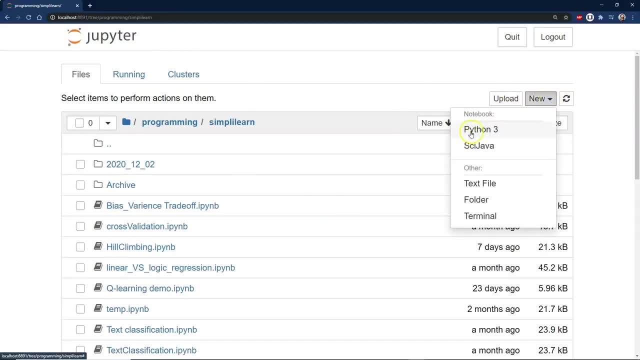 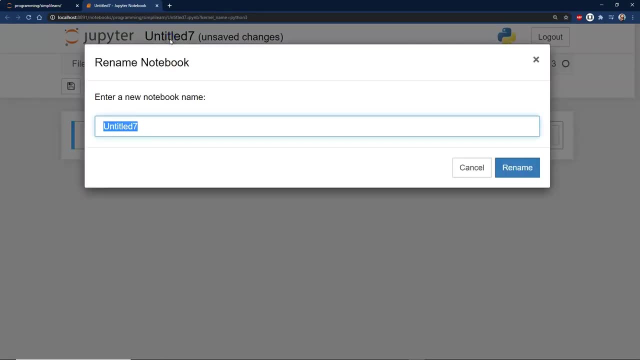 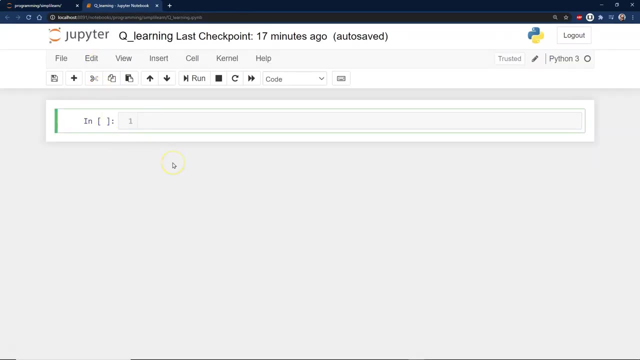 in our Jupiter notebook, which has the kernel loaded with Python 3, we'll go ahead and create a new Python 3 folder in here and we'll call this Q learning. and to start this demo, let's go ahead and import our numpy array. we'll just 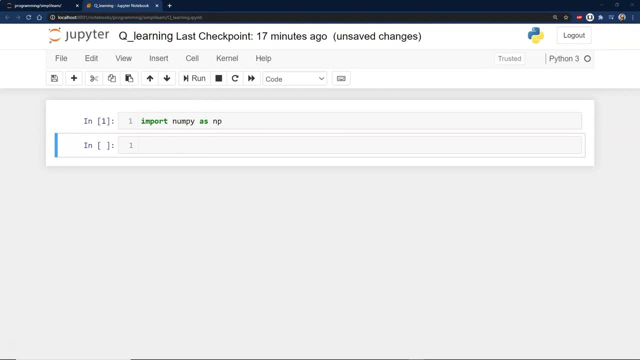 run that, so it's imported and, like a lot of these model programs, when you're building them you spend a lot of time putting it all together and then you end up with this really short answer at the end, and we'll take a look at that as we. 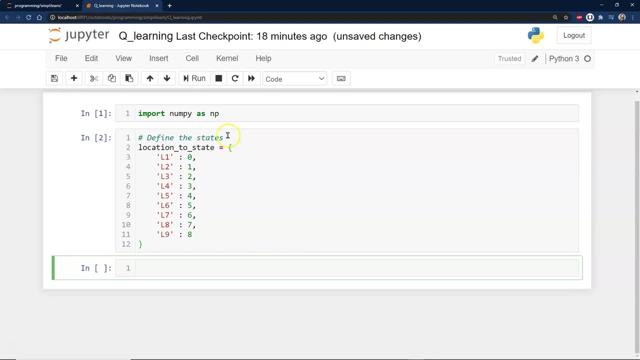 come into it. so we go ahead and start with our location to state. so we have L1, L2, these are our eight and nine, and then, of course, the state is going to be zero. one, two, three, four. it's just a mapping of our location to a integer on there, and then we have our actions. our actions are simply: 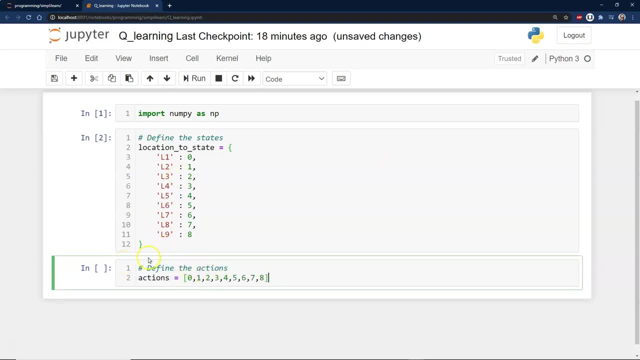 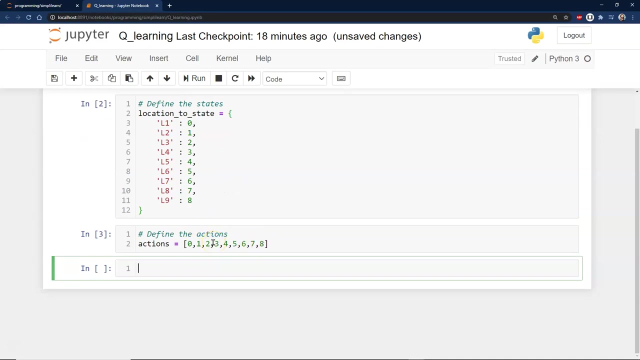 moving from one location to another. so I can go to. I can go to location zero, I can go to location one, two, three, four, five, six, seven, eight. so these are my actions, I can choose. these are the locations of our state and, if you remember, earlier I mentioned that the limitation is that you, you don't want to put in a continually growing. 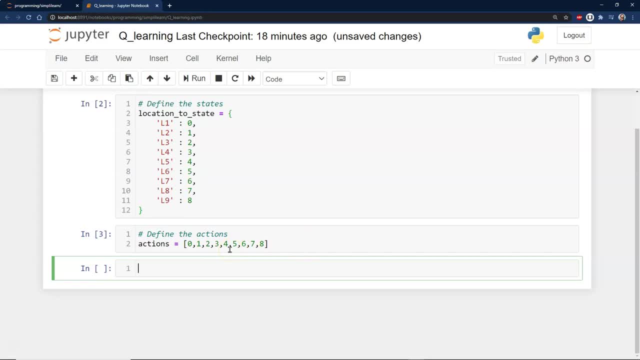 table, because you can actually create a dynamic Q table where you continually add in new values as they arise, because if you have float values it just becomes infinite and then your memory and your computer is gone or you know it's not going to work. at the same time, you might think well that 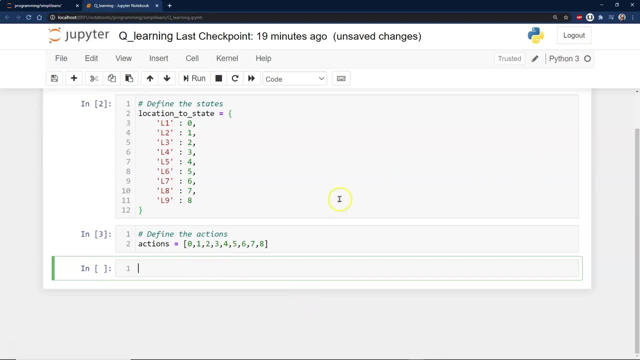 kind of really limits the the Q learning setting set up, but there are ways to use it in conjunction with other systems and so you might look at. uh, well, I do. I've been doing some work in stock and one of the questions that comes out is to buy or sell the stock. 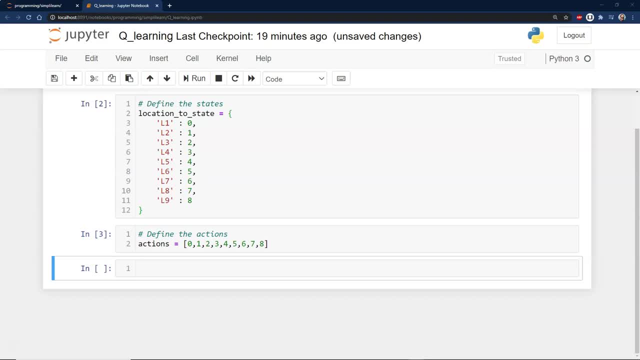 and the state coming in might be, you might take it. you can create what's called buckets, where anything that you predict is going to return more than a certain amount of money- The error for that stock that you've had in the past. you put those in buckets and suddenly you start creating these buckets. 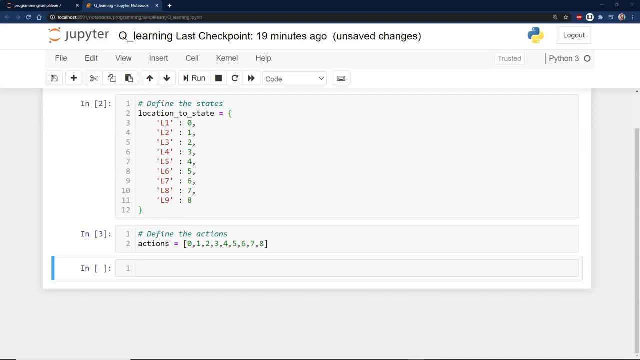 you realize you do have a limited amount of information coming in. You no longer have a float number. You now have bucket 1,, 2,, 3, and 4. And then you can take those buckets, put them through a Q-learning table and come up with the best action. Which stock should I buy? 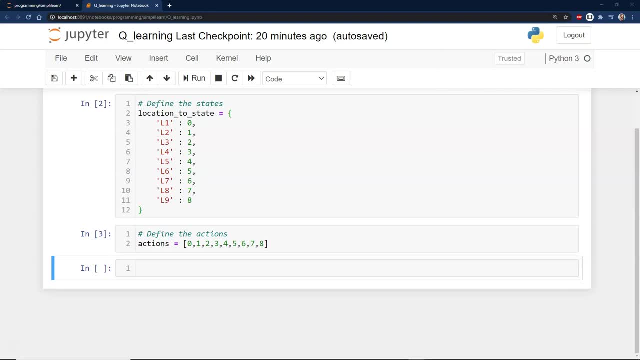 It's like gambling. Stock is pretty much gambling. if you're doing day trading, You're not doing long-term investments, And so you can start looking at it like that. A lot of the current feeds say that the best algorithms used for day traders, where you're doing it on your own, is really to ask the question. 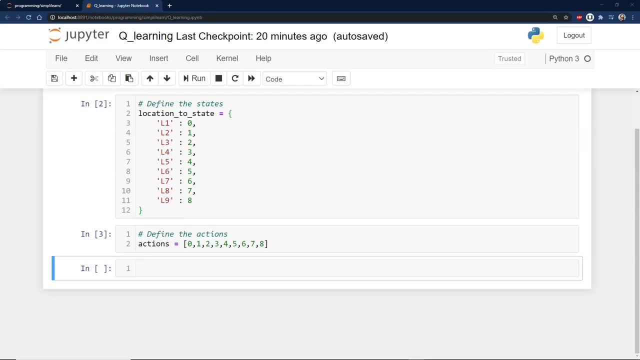 do I want to trade the stock, Yes or no? And now you have it in a Q-learning table and now you can take it to that next level And you can see where that can be a really powerful tool at the end of doing a. 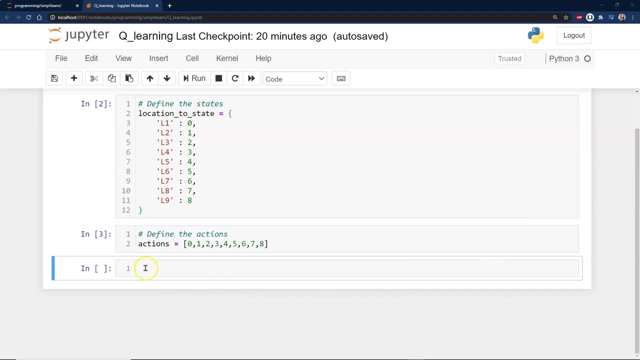 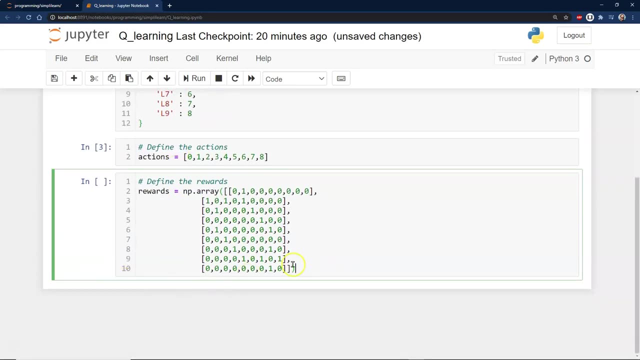 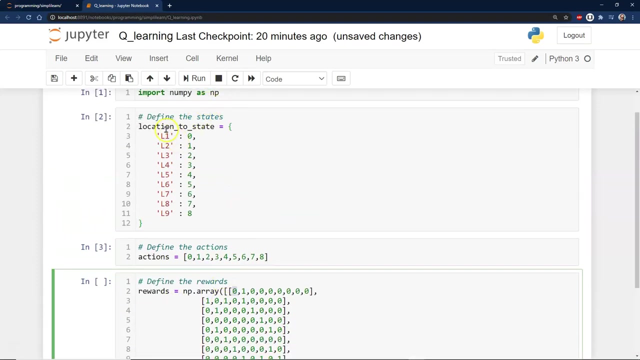 basic linear regression model or something. What is the best investment? And you start getting the best reward on there. And so if we're going to have rewards, these rewards we just create. It says basically: if you're, this should match our Q-table, It's going to be. you have your state. 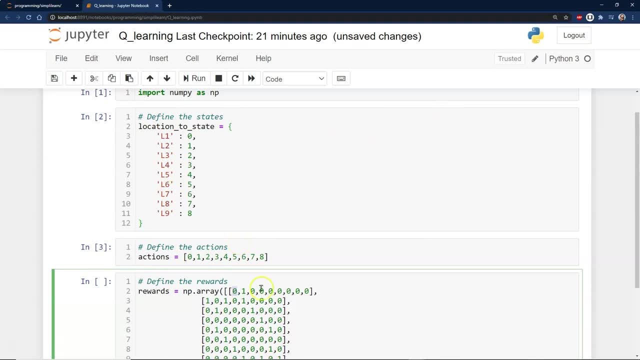 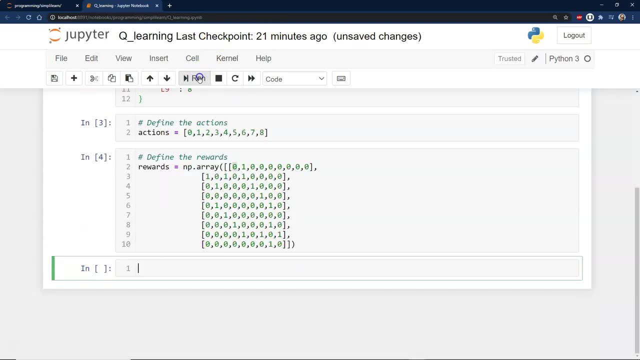 and you have your action across the top, if you remember, from the dog, And so we have whatever state we're in going down, and then the next action and what the reward is for it And, of course, if you were actually doing something more connected, your reward would be based on. 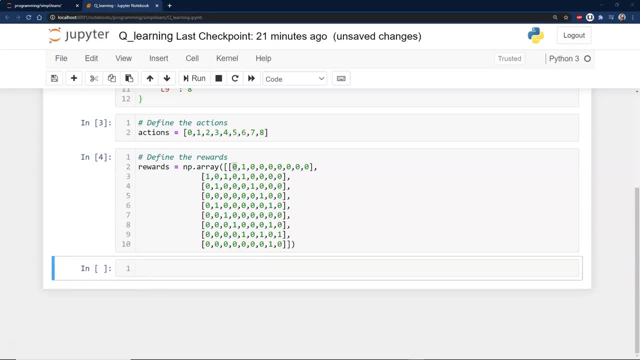 the actual environment it's in. And then we want to go ahead and create a state to location so we can map the indexes. So, just like we defined our rewards, we're going to go ahead and do state to location. And you can see here it's a dictionary. 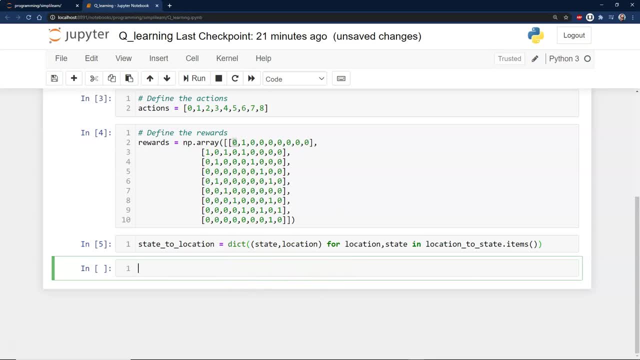 setup for location state and location to state With items, And we also need to define what we want for learning rates. You remember we had our two different rates as far as like learning from the past and learning from the current, So we'll go ahead and set those to .75 and the alpha set to .9.. 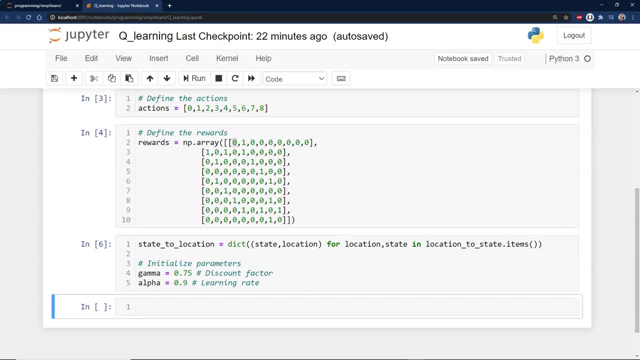 And we'll see that when we do the formula And, of course, any of this code, send a note to our Simply Learn team. They'll get you a copy of this code on here. Let's go ahead and pull. There we go. 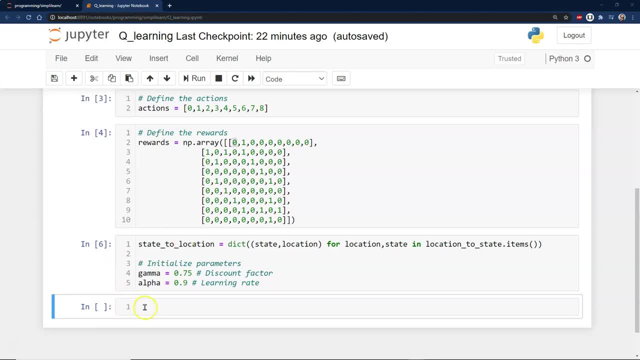 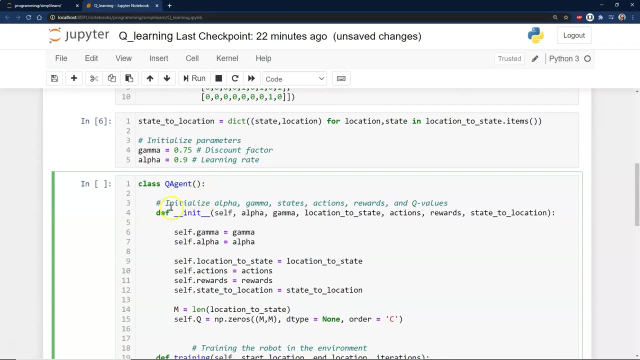 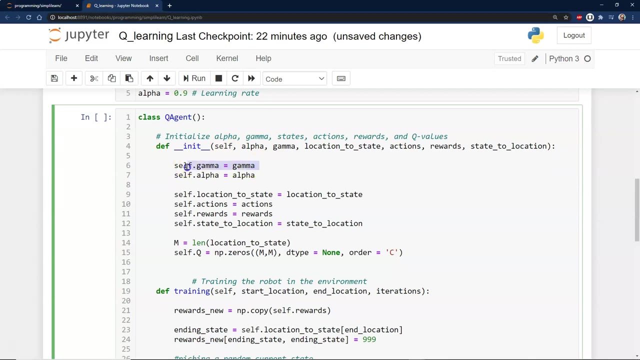 The next two sections, Since we're going to keep it short and sweet. Here we go. So let's go ahead and create our agent. So our agent is going to have our initialization, where we send it all the information We'll define ourself. gamma equals gamma. We could have just set the gamma rate down here. 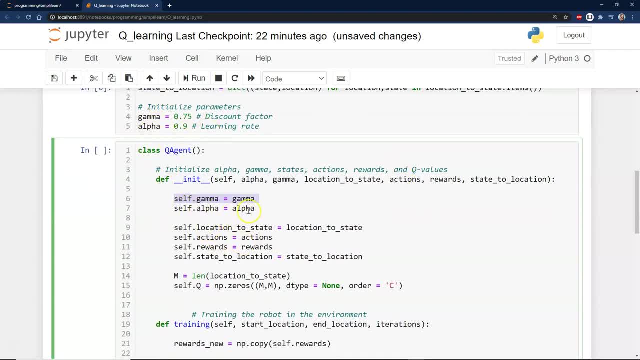 instead of submitting it. It's kind of nice to keep them separate, because you can play with these numbers: Ourself, alpha. Then we have our location state. We'll set that in here. We have our choice of actions. We're going to go ahead and just. 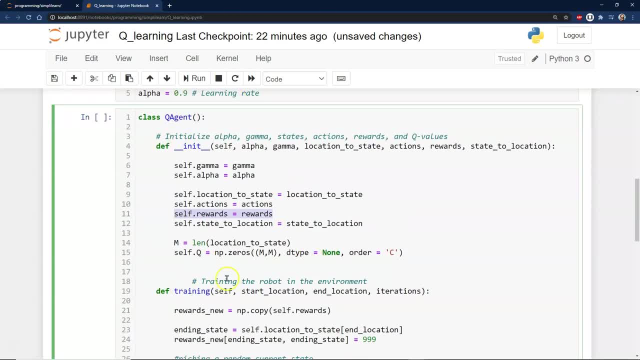 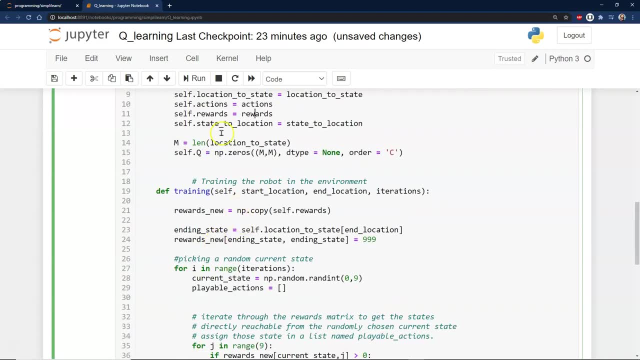 embed the rewards right into the agent, So obviously this would be coming from somewhere else instead of from self-generated. And then a self state to location equals our state to location dictionary. And we go ahead and create a Q learning table, And I went ahead and 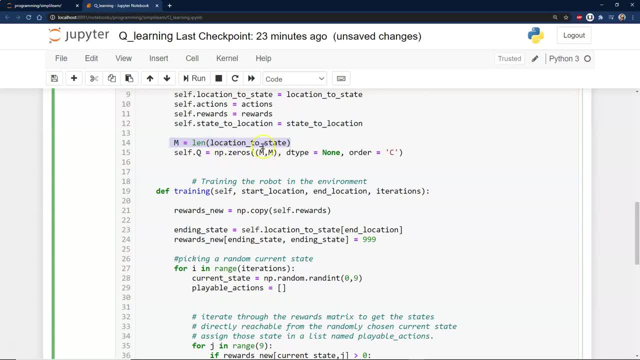 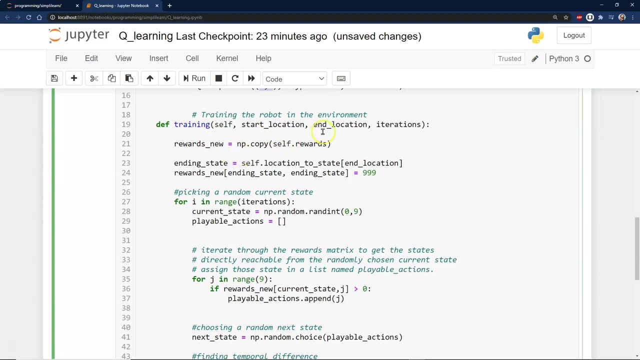 just set the Q learning table up to 0 to 0. What the setup is, Location to state How many of them are there. This just creates an array of 0 to 0 setup on there And then the big part is the training. We have our rewards: new equals. 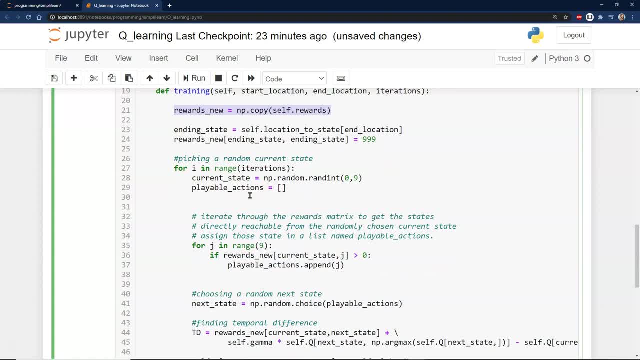 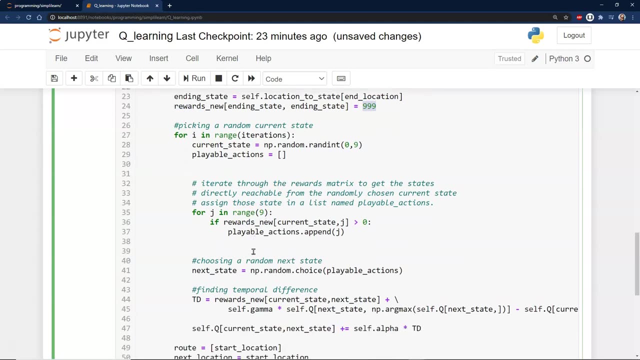 a copy of selfrewards. Ending state equals the self location state in location. So this is whatever we end up at. Rewards: new equals ending state plus ending state equals 999.. Just kind of goes to a dead end And we start going through. 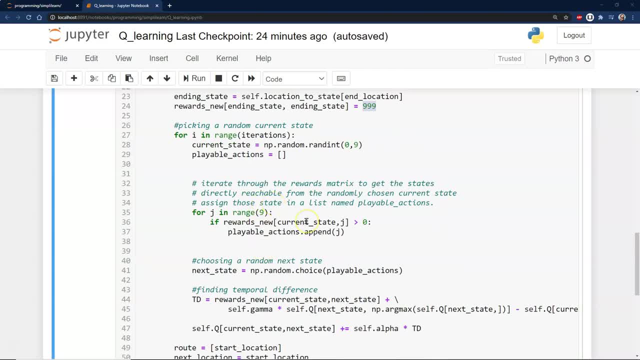 iterations And we'll go ahead. Let's do this. So this, we're going to come back and we're going to call it on here. Let me just erase that, Switch it to an arrow. There we go. So what we're doing is we're. 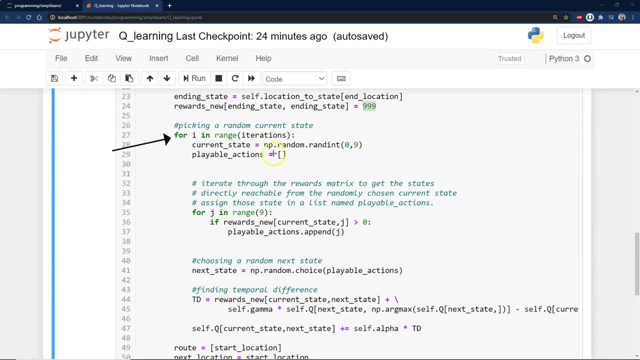 going to send in here to train it. We're going to say, hey, I want to iterate through this a thousand times and see what happens. Now this part would actually be: instead of iterating, you might have your external environment and they're going back and forth and you iterate through outside of here. But just for 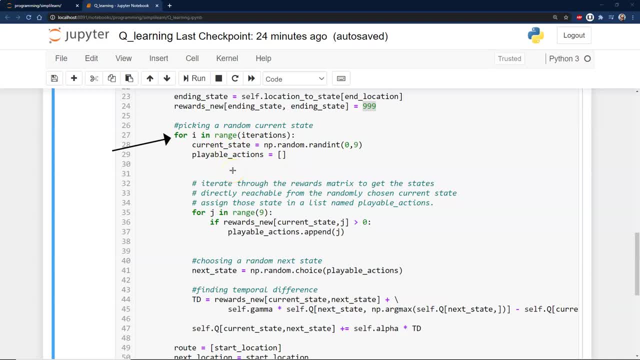 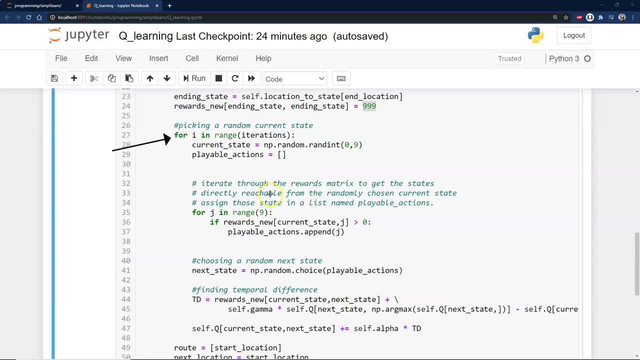 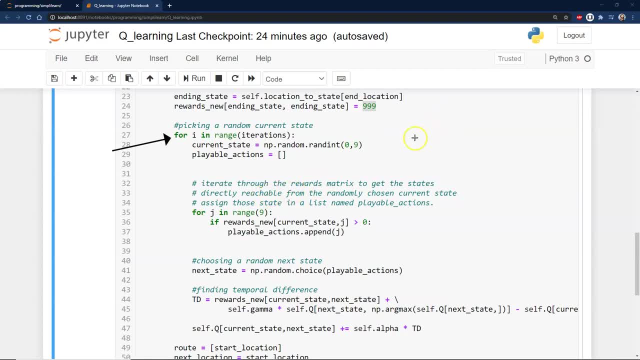 And then we want to go ahead and pick a random state to start with. That's what's going on here. You have to start somewhere, And then you have your playable actions. We're going to start with just an empty thing for playable actions and we'll fill that up. So that's what choices I have, And so we're going. 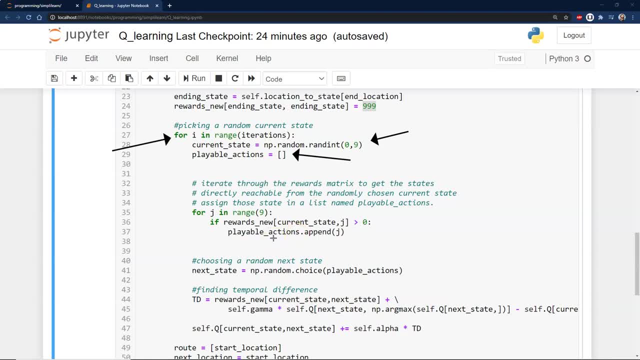 to iterate through the rewards matrix to get the states Directly reachable from the randomly chosen current state. Assign those states to a list named playable actions, And so you can see, here we have a range 9. I usually use lengths of whatever I'm looking at, which is our. 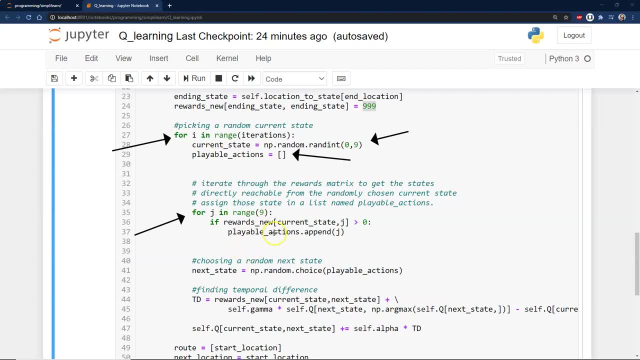 locations or states as they are. We have a reward. So we want to look at the current the rewards. the new reward is our, is in our chart here of rewards, underscore new current state plus J, J being what is the next state? we want to try, And so we go ahead and do our. 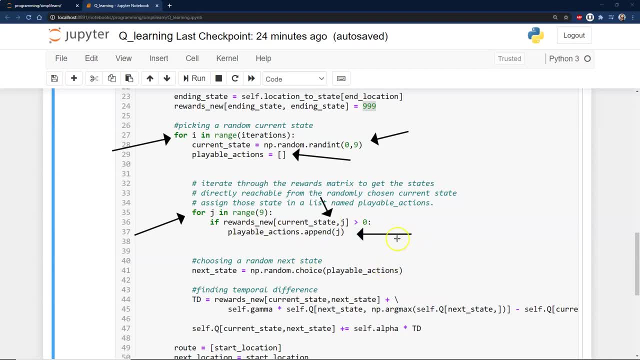 playable actions and we append J, And so what we're doing is we're randomly trying different things in here to see what's going to generate a better reward, And then, of course, we go ahead and choose our next state. So we have our random 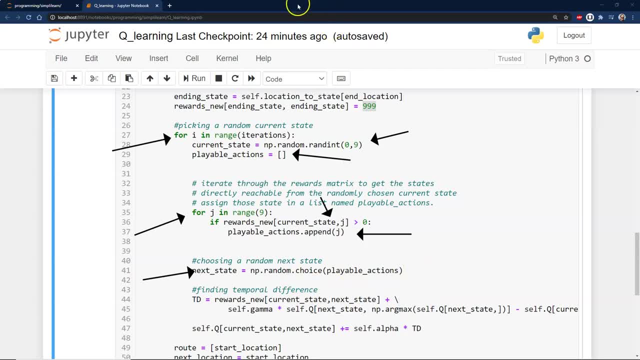 choice, playable actions And, if you remember, I mentioned- on this- let me just go ahead and do a free form- When we were talking about the next state. this right here just does a random selection. Instead of a random selection, you might do something where, whatever the best selection is, which. 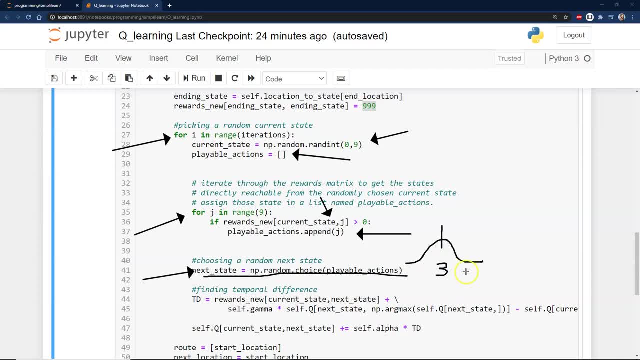 might be option 3 here And then- so you can see- that it might use a bell curve, and then option 2 over here might have a bell curve like this, And we start looking at these averages and these spreads, or we can just add them all. 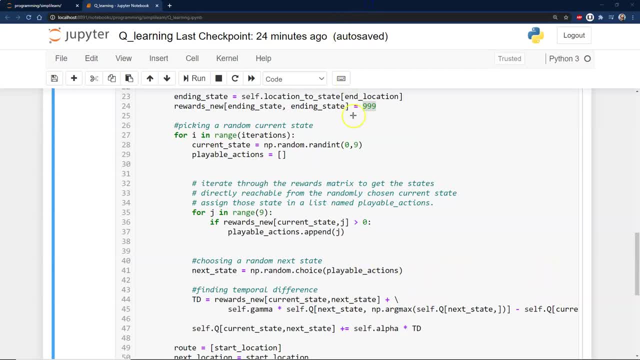 together and pick the one that kind of goes in all of those. So those are some of the options we have in here. We just go with a random choice. That's usually where you start to play with it, And then we have our rewards section down here. 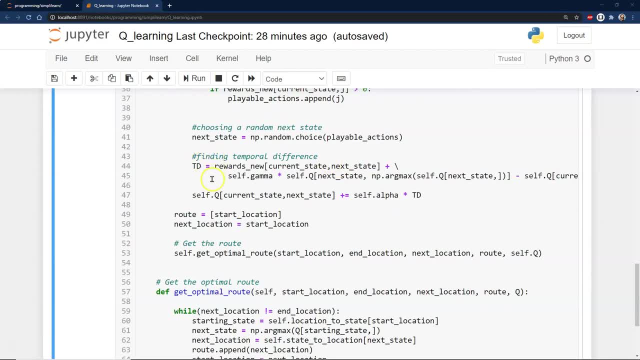 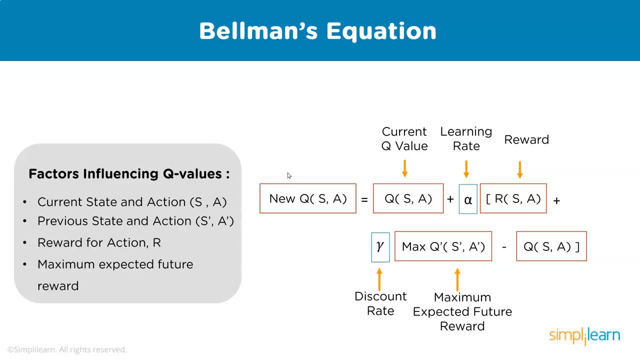 And so we want to go ahead and find- well, in this case, a temporal difference. So you have your rewards new, plus the self gamma, And this is the formula we were looking at. This is Bellman's equation here. So we have our current value, our 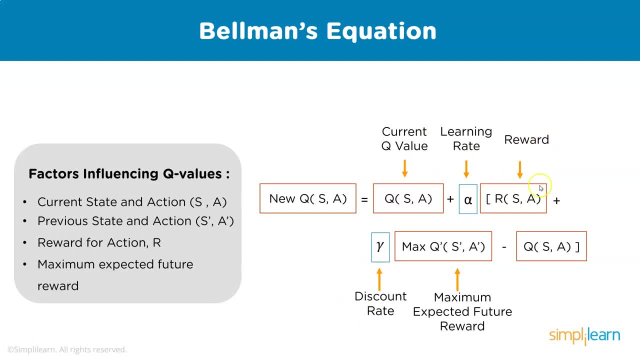 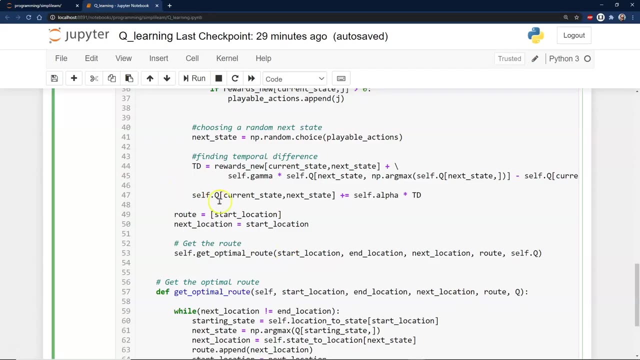 learning rate, our discount rate involved in there, the reward system coming in for that, And we can add it all together. This is, of course, our maximum expected future setup in here. So this is all of our Bellman's equation that we're looking at here, And 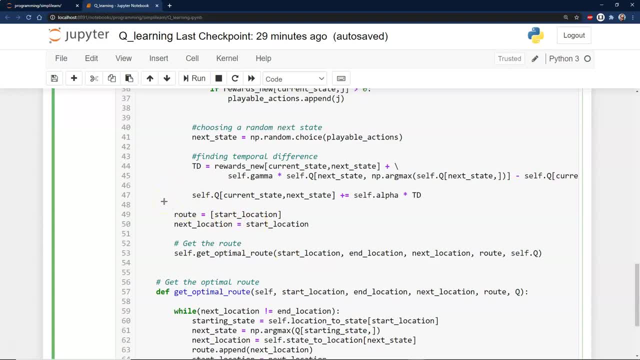 then we come up in here and we update our cue table. That's all. this is on this one. That's right here We have self cue- current state, next date, and we add in our alpha because we don't want to do that. 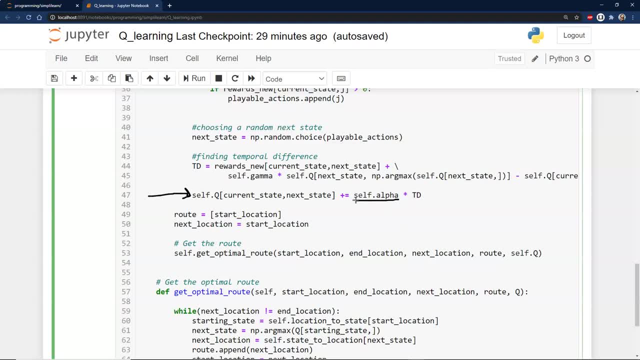 We don't want to train all of it at once, in case there's slight differences coming in there. We want to slowly approach the answer And then we have our route equals the start location and next location equals start location. So we're just incrementing. We took a step forward And then finally remember I was- 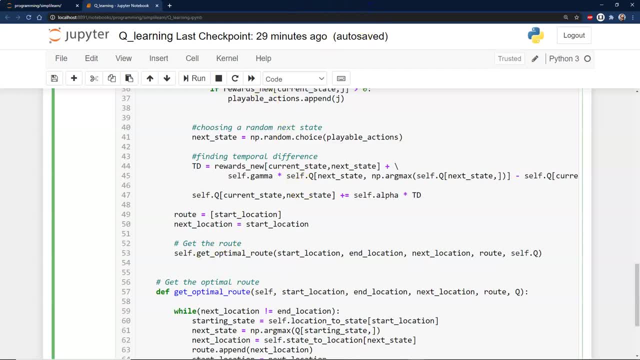 telling you how we're going to do all this and just have some simple thing at the end or just generates a simple path. We're going to go ahead and get the optimal route. We want to find the best route in here, And so we've created a definition for the optimal route down here. Just scroll down. 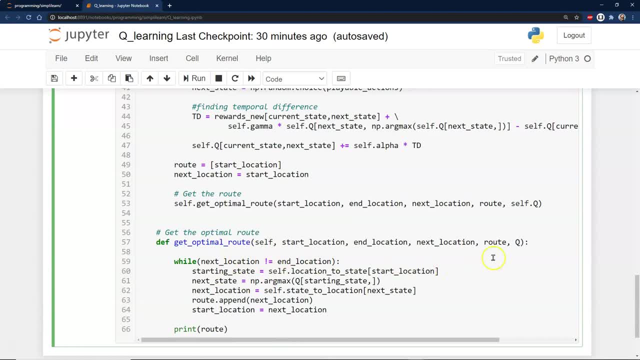 for that And we get the optimal route. We go ahead and put the information in, including the cue table: self start location in location, next location, route cue And it says while next location is not equal to in location. so while we can, 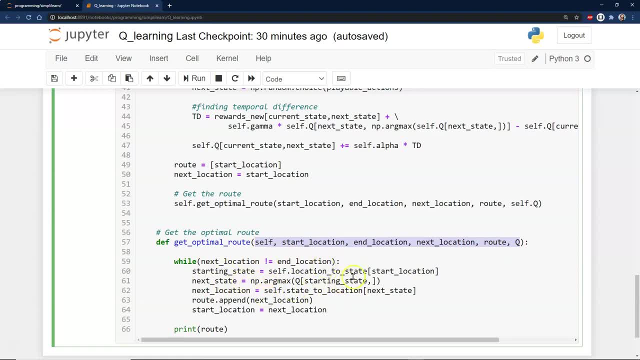 still go. our start location equals self location to state start location, So we already have our best value for the start location. The next location equals the start location. So we're going to go ahead and look at the cue table and say, hey, what's the next one with the best value? 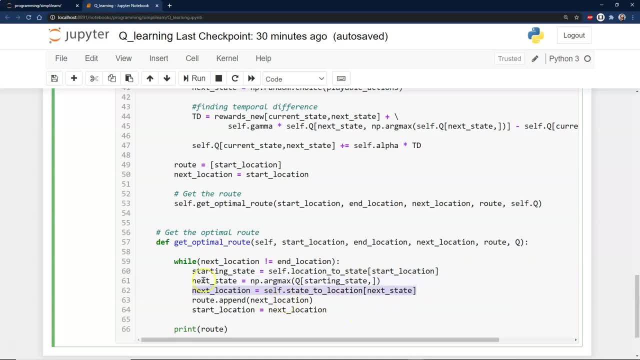 And then the next location. we go ahead and pull that in and we just append it. That's what's going on down here. And then our start location equals the next location And we just go through all the steps And we'll go ahead and run this. 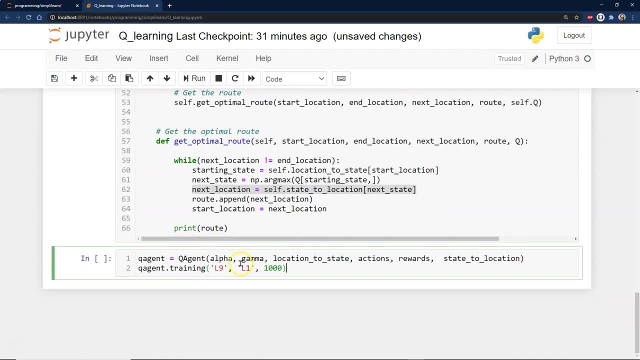 And now that we have our cue table, our cue agent loaded, we're going to go ahead and take our cue agent, load them up with our alpha gamma that we set up above, Along with the location, step, action, reward, state to location. And our goal is: 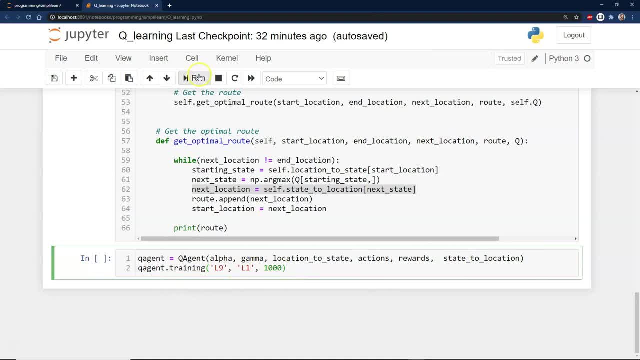 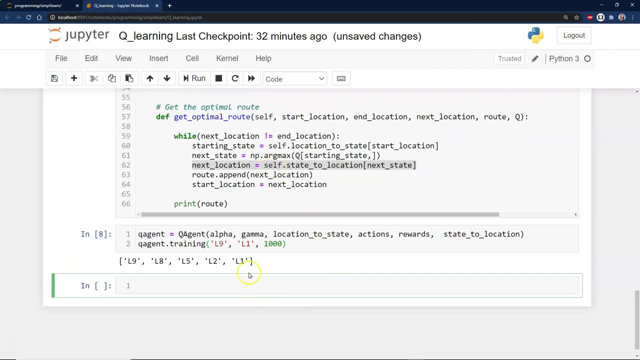 to plot a course between L9 and L1.. And we're going to go through a thousand iterations on here And so when I run that it runs pretty quick. Why is this so fast If you've been running neural networks and you've been doing all these? 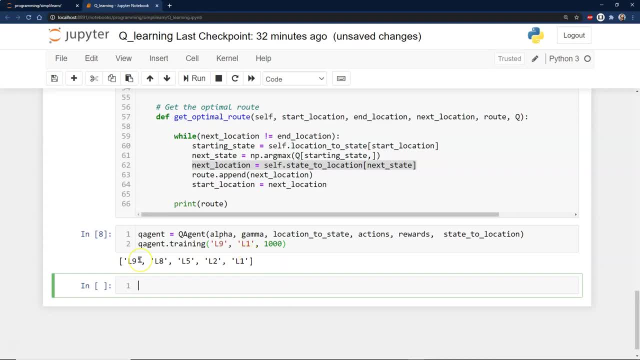 other models. you sit here and wait a long time. Well, we're a very small amount of data. These are all integers. These aren't float values. The math is not heavy on the processing end And this is where cue tables are. so 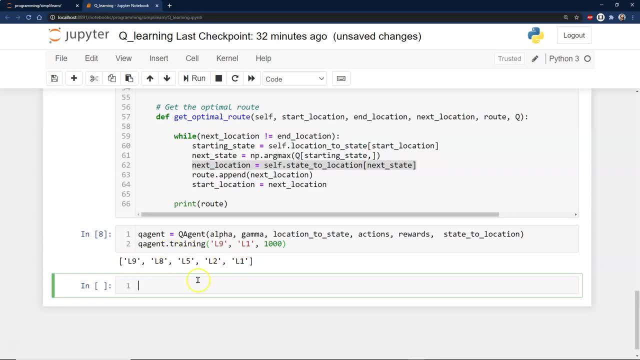 powerful. If you have a small amount of information coming in, you very quickly get an answer off of this, even though we went through it a thousand times to train it, And you'll see here we have L9,, 8,, 5,, 2, and 1.. And that's based on our reward. 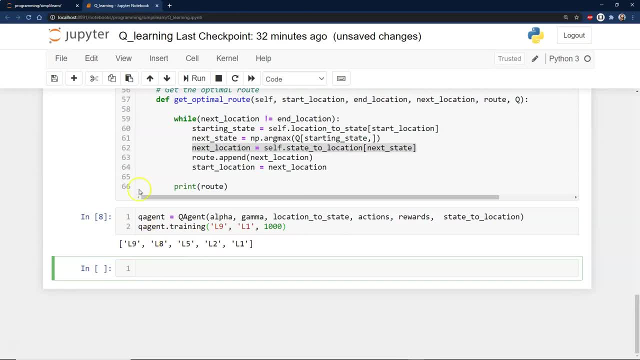 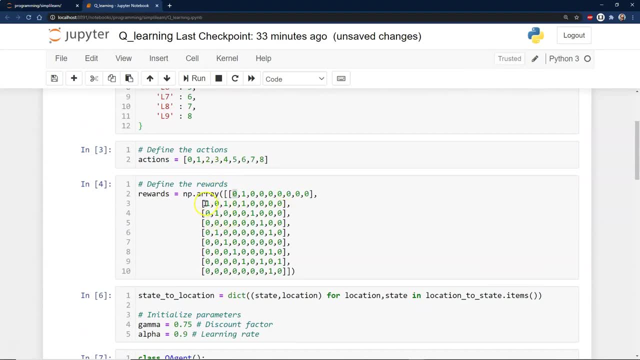 table we had set up on there And this is the shortest path going between these different setups in here. And if you remember, on our reward table, you can see that if you start here you can go to here. There's places you can't go. That's how this reward table was set up, So I can.